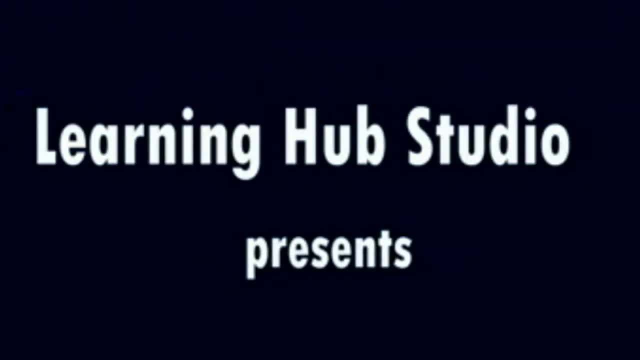 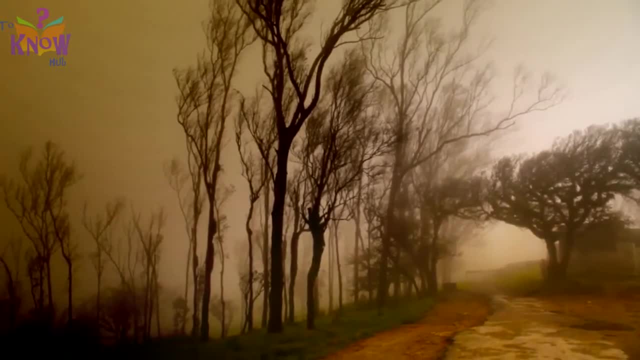 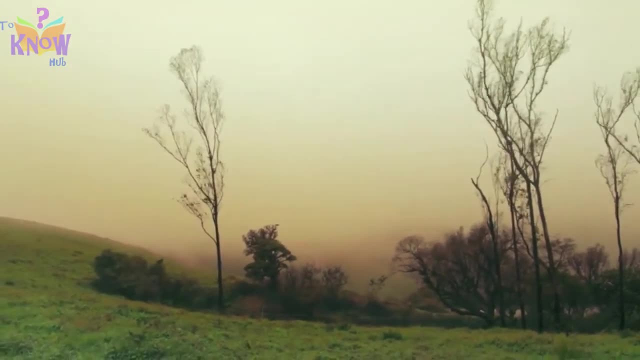 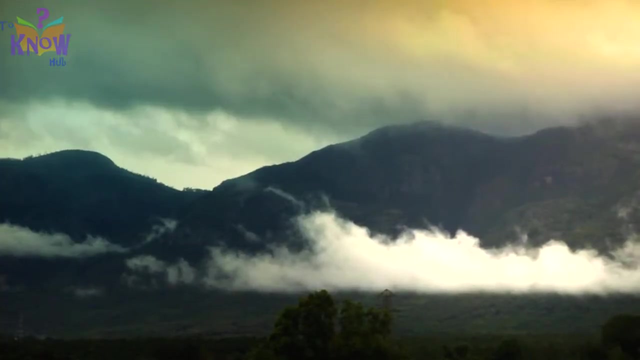 Now, most of us put all the blame on global warming whenever it comes to climate change, but there are many things more which are making those cyclones famine, which are responsible for those heat wave, those cold wave. so science is important, but other than science, geography has gained enough importance. 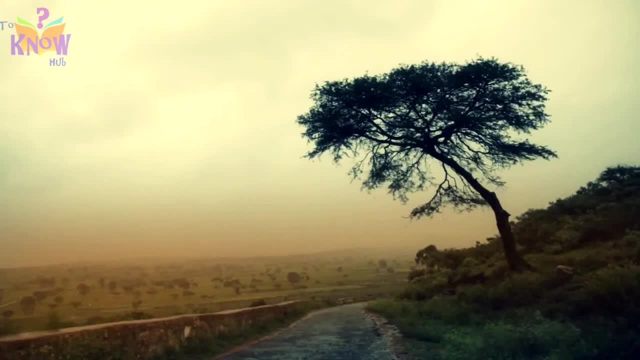 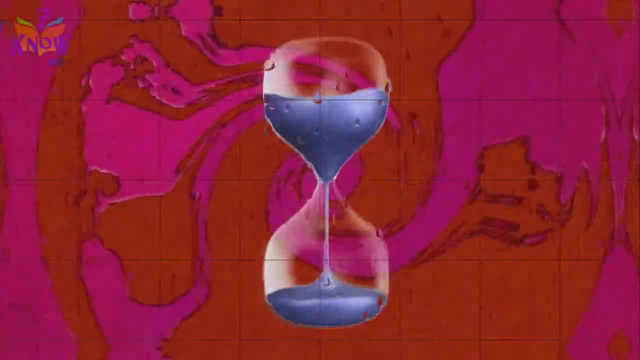 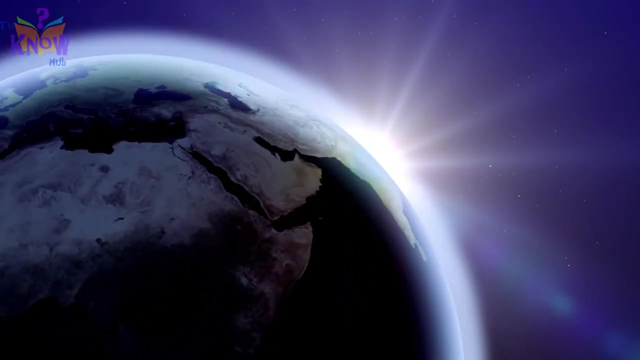 in today's time, because we need to understand exactly what is wrong with this world, exactly what is wrong with our climate. so let's start with the geography series. so we'll be starting with physical geography series. we will go deeper and deeper. we know about the atmosphere, so so 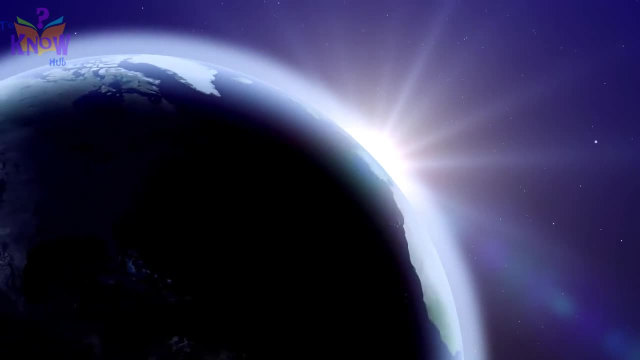 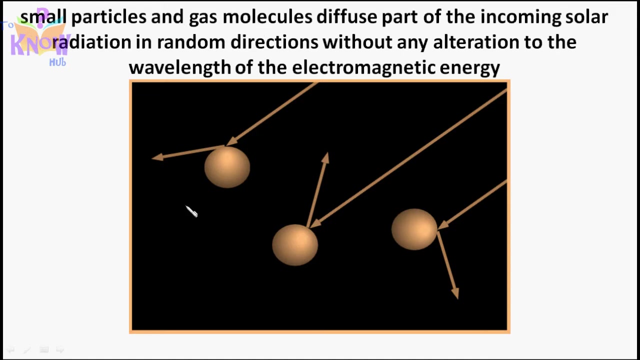 let's now understand exactly what happened to the solar radiation which is thrown towards the earth. now three things happen to the solar radiation. first is scattering. what is scattering? the process of scattering occurs when small particles or gas molecules diffuse part of incoming solar radiation in random direction, means they absorb. 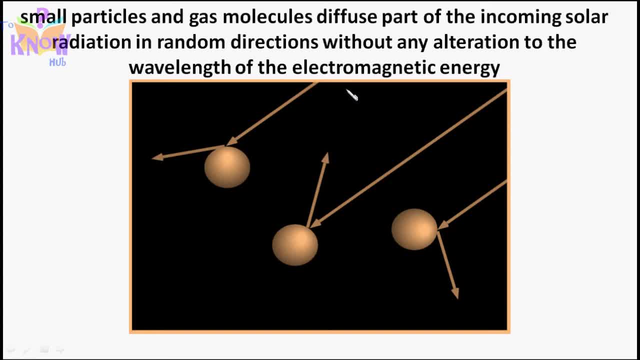 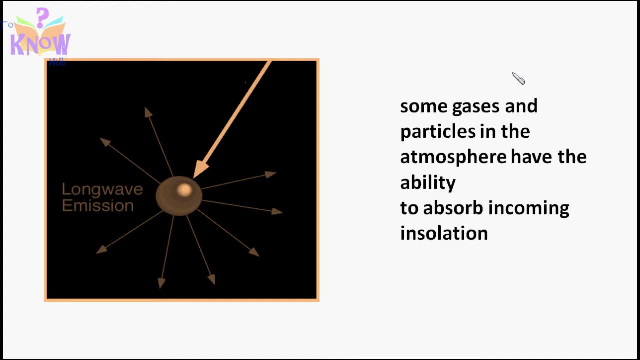 the solar radiation, they start vibrating and and release the wave in every direction. so they are actually scattering the wave, so it is called scattering. now only few portion of this scattered energy actually reaches the earth. what is absorption in this process? we know that molecules or particles absorb radiation. but here, after absorbing radiation, they release the energy, so they first. 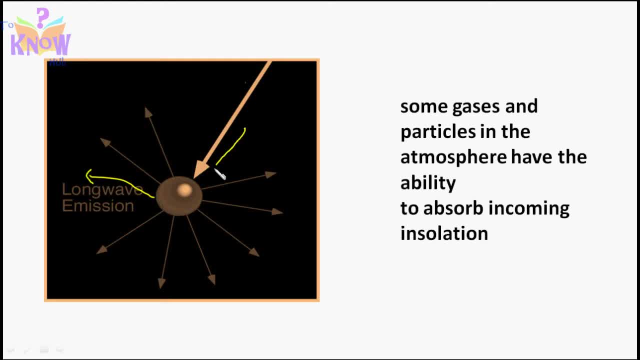 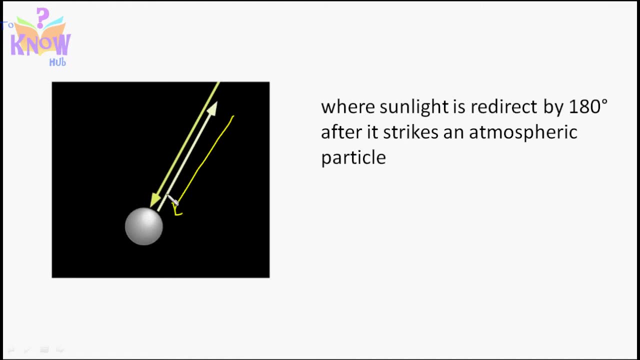 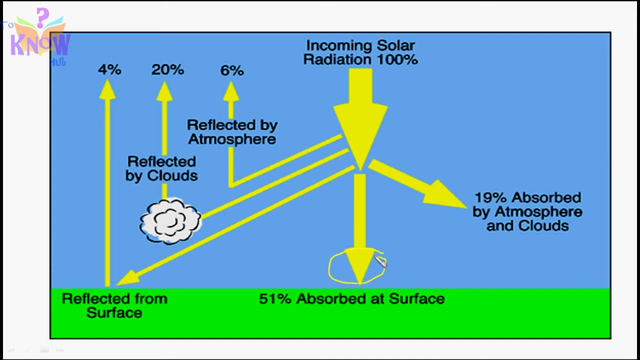 absorb, then release the energy, but most of this released energy goes back to space. and the third thing happened, which is reflection. as the name implies, molecules in atmosphere reflect solar energy, that is, solar radiation. clouds reflect solar energy. only 51 percent of the solar radiation reaches the earth. so what happened to rest of it? 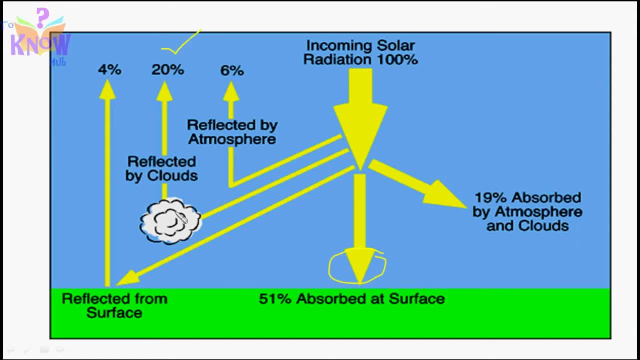 around 20 percent get reflected by the cloud and six percent gets reflected by the atmosphere. around four percent is reflected from the surface. when this solar radiation falls on snow or glaciers, they reflect back. so around four percent of the solar radiation reflect back from the surface. we lose around the 30 percent of the solar radiation in these three processes. 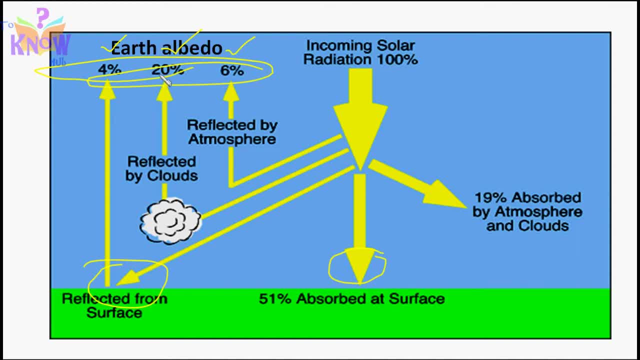 now, reflectivity of the surface is often described as albedo. now earth's average albedo reflectance from both surface and the atmosphere is about 30 percent, twenty percent by cloud, six percent by other elements of the atmosphere and four percent is the surface. so thirty percent. 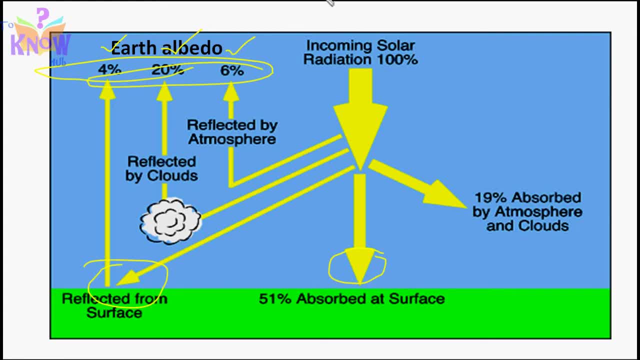 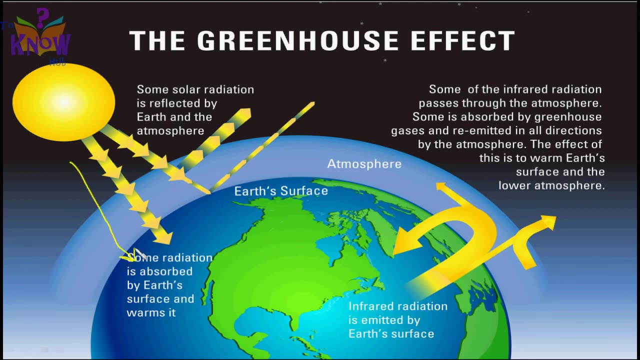 albedo: thirty percent reflectivity. now nineteen percent of the solar radiation get absorbed by the atmosphere. now let's come to greenhouse effect. we just came to know that fifty one percent of the solar radiation actually reaches the surface. surface absorbs it and surface also radiate back. 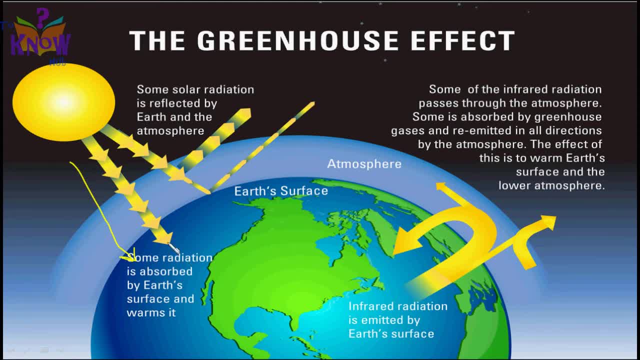 now. surface absorbs the short wavelength solar radiation but it radiates back as long wavelength radiation. greenhouse gases absorb long wavelength. after absorbing radiation they release the energy. so they first absorb, then release the energy. so what they do is they release back those long wavelength to surface every time surface. 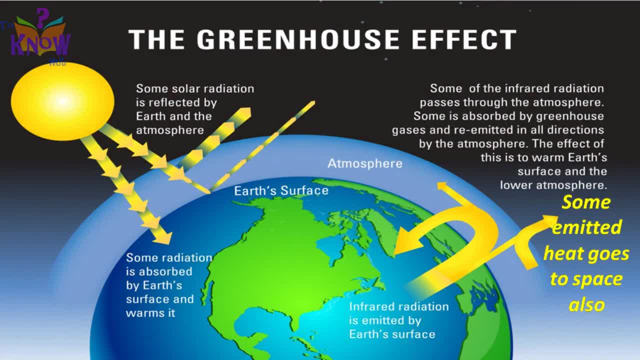 absorbs some heat, it radiates back the ninety percent of it as long wavelength. this keeps happening and happening and the heat remain trapped in our atmosphere for a long time. accumulation of this heat over time can actually increase the temperature of earth, but, as you know, that temperature hasn't increased by 10 degrees celsius. of 50 degrees celsius, that didn't happen. 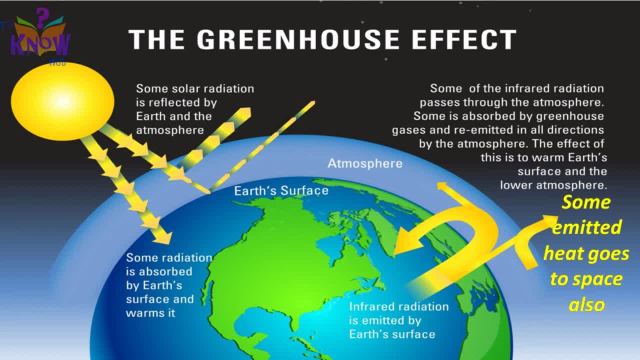 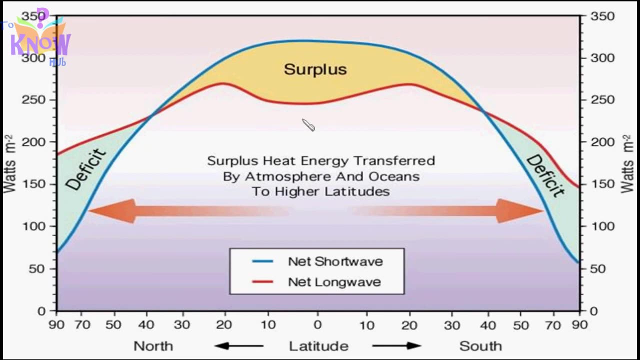 it increased by full degree celsius. hold your horses. the explanation is not over. we may need to go deeper, but later. so exactly what happened? if we look at this figure, we can see surface, absorb short wavelength and release long wavelength, and near the equator, in the tropical region. 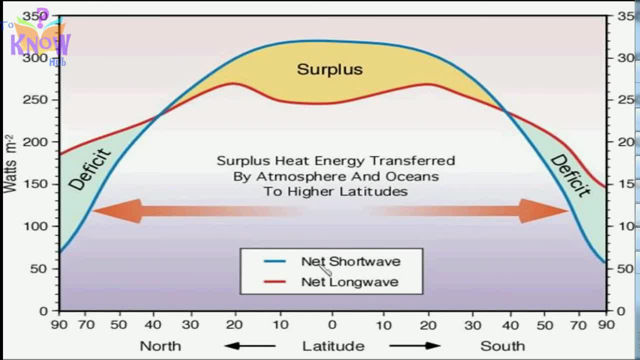 there is lots of solar radiation available, so so surface absorbs a lot. it doesn't radiate back a little. we get a lot of heat similar to the force of the surface, so we get a net increase in everything. so we get a net increase in energy. but as we move towards the pole, the solar radiation 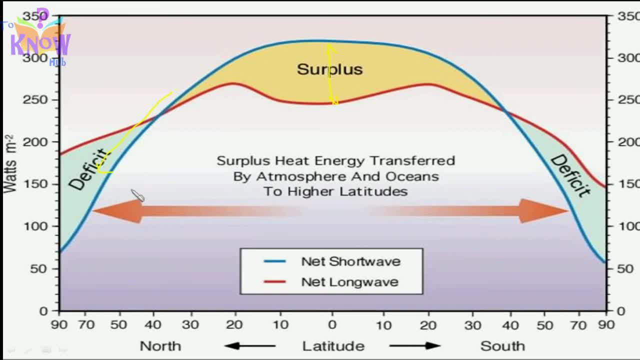 decreases the surface, absorbs less heat, but it radiates almost all of it. it also loses some extra energy because of longer nights. we get a deficit because difference of incoming and outgoing energy is negative. so energy is basically or no less than 2-3 times. so we get space. so we get space. so we have more energy, we get energy. 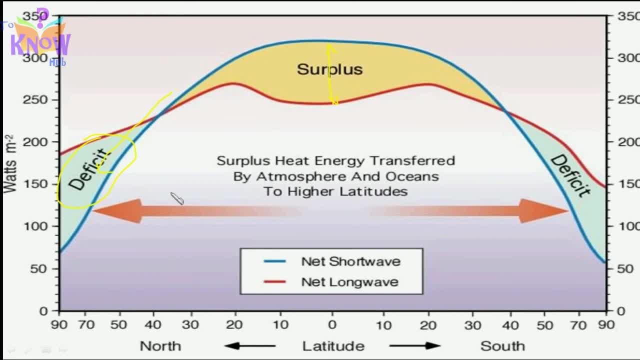 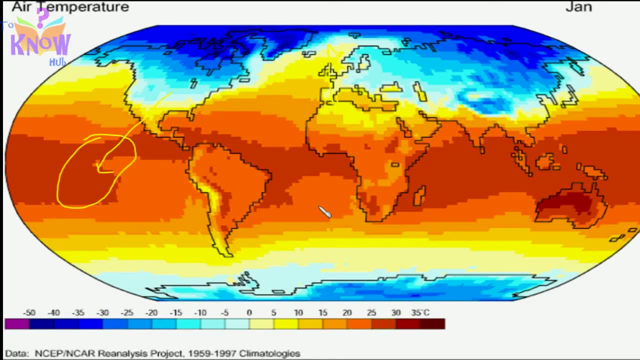 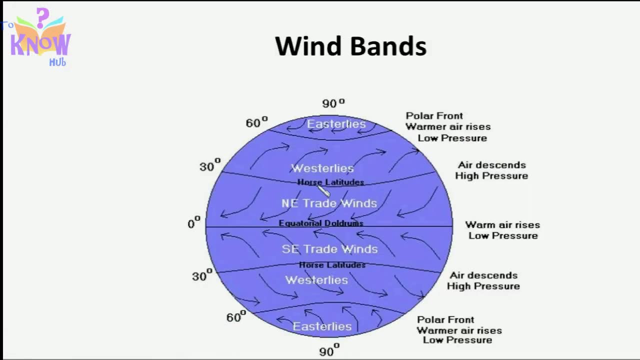 so we get a deficit. we get a deficit at higher latitude and we have a surplus near the equator. so this difference of energy label actually creates the wind. this difference of energy is very important. it gives us the weather. let's summarize what happened to the solar radiation: 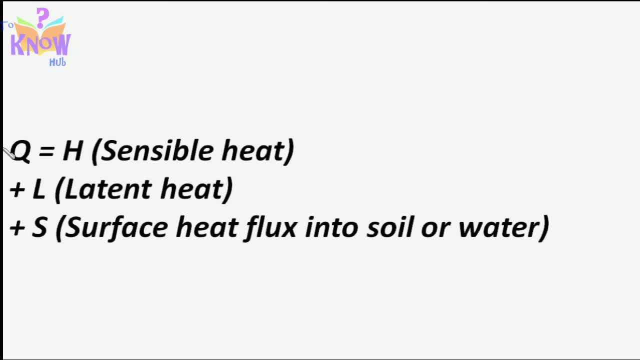 in short, very short. if q is the energy that somehow reaches the surface, that is, the 50 percent of the solar energy, we can divide it into three parts: one, the sensible heat, two, the latent heat and three, the surface heat flux into soil and water. sensible heat: it is part of the heat that 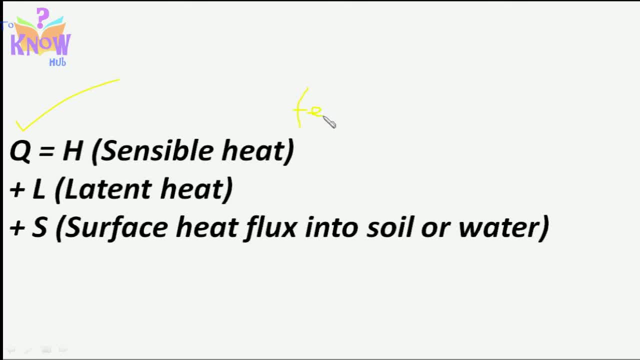 we can feel. so if you are standing on ground bare feet and you are feeling the heat- the ground is hot- then you are actually feeling the sensible heat and the latent heat. we know when, when liquid turn into solid, it releases latent heat, and for solid to turn into liquid it needs latent heat. 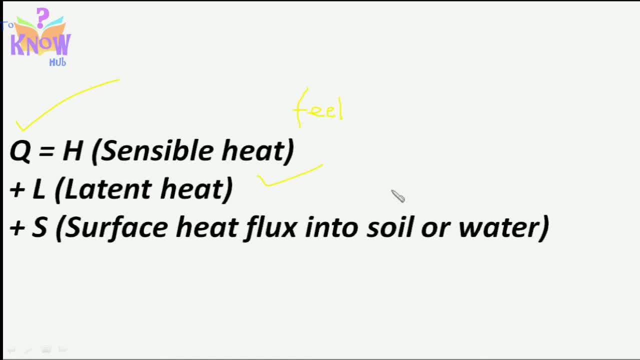 so latent heat. latent heat flux moves energy globally when solid liquid and gas interchanges form. and the third is surface heat flux into soil and water. as you saw, the 10 percent deficit every time. as the specific heat of the water is very high, it also absorbs lot of heat. what happened to this heat is they get transferred. 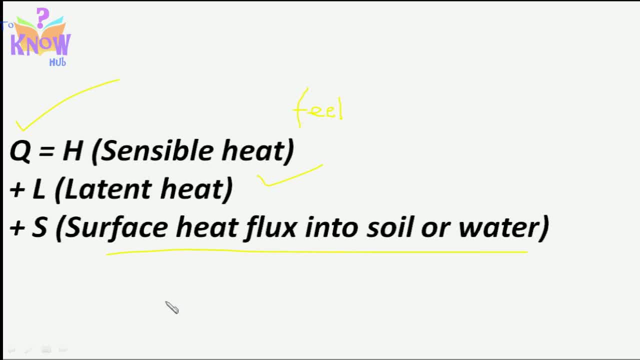 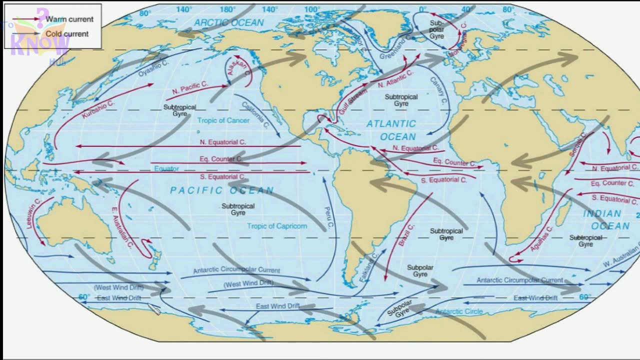 inland they get transferred to conduction process deeper and deeper, and in water they get transferred through convection process, and in water this absorption of heat is more near the equator region and less in the higher latitude, so we get a temperature gradient difference of temperature and because of this difference of temperature we get ocean current. so that's all for now. 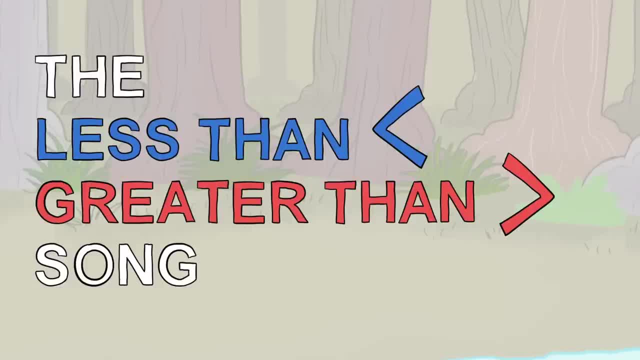 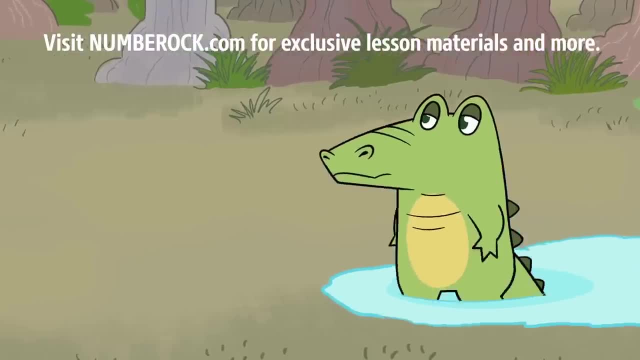 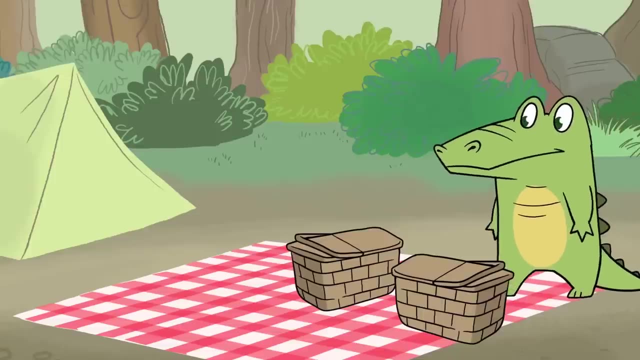 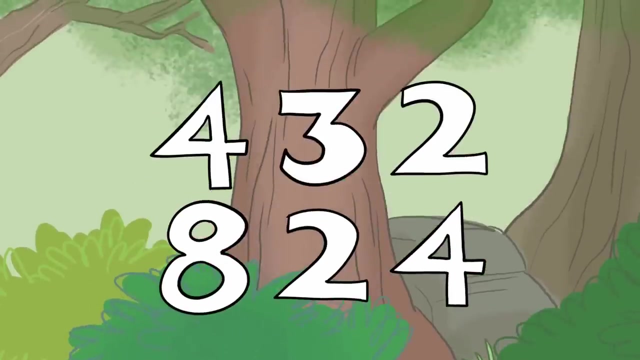 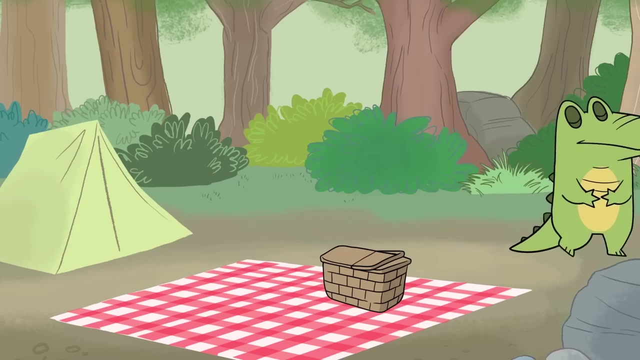 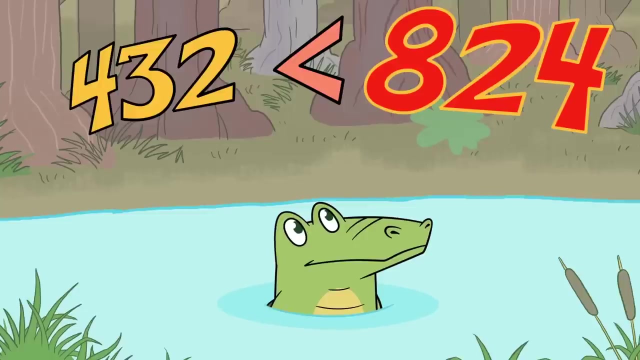 432 and 824.. The gator eats the one that's worth more. He looks at the place values from left to right. It's the greatest hundreds place, so he takes a big bite. Uh-huh, The hungry alligator eats the number that's greater. The number that is least is never part of his speech. 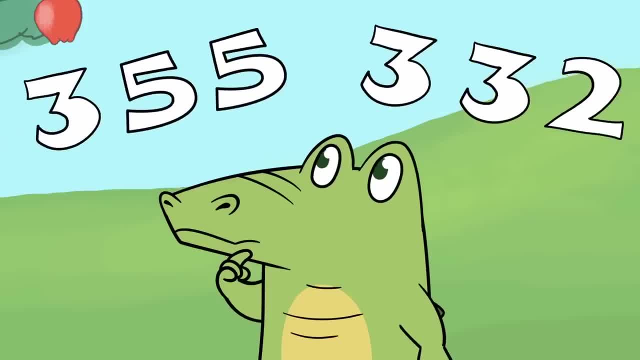 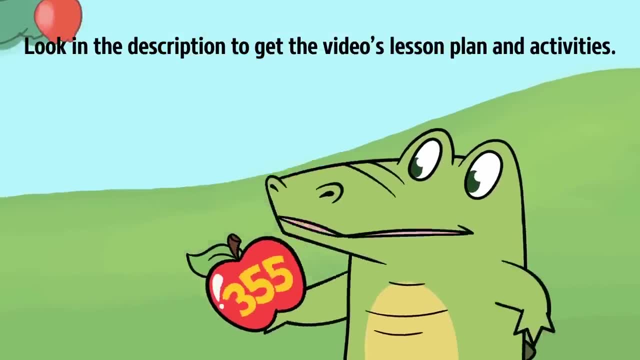 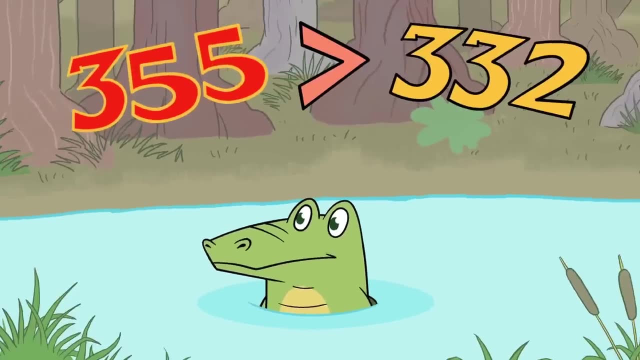 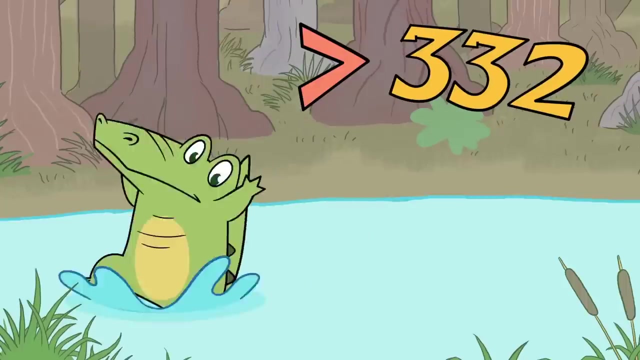 355 and 332.. The gator needs to eat the one with the greater value. He looks at the place values from left to right. 5 is the greatest tens place, so he takes a big bite. Uh-huh, The hungry alligator eats the number that's greater. The number that is least is never part of his speech. 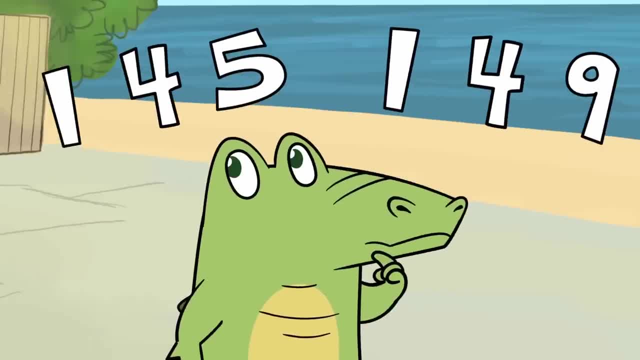 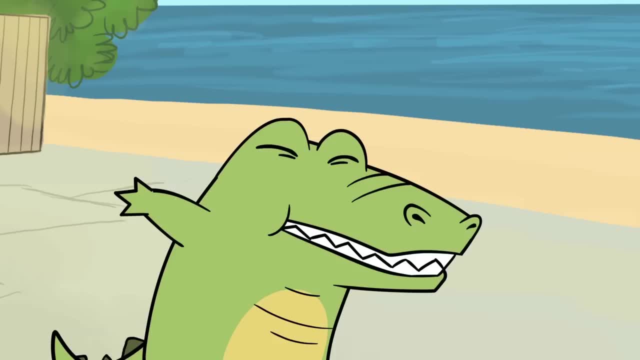 145 and 149.. The gator needs the greater value on the number line. He looks at the place values from left to right. 9 is the greatest ones place, so he takes a big bite. Uh-huh, The hungry alligator eats the one that's worth more. He looks at the place values from left to right. 9 is the greatest ones place, so he takes a big bite.